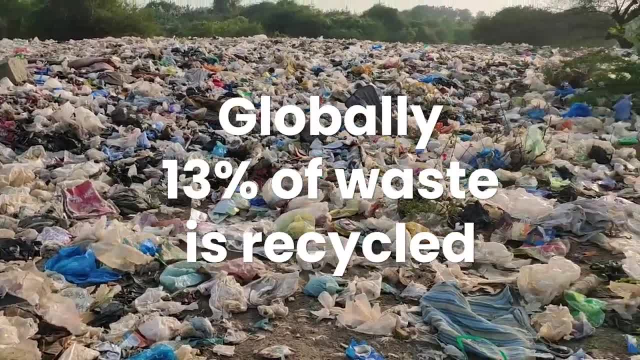 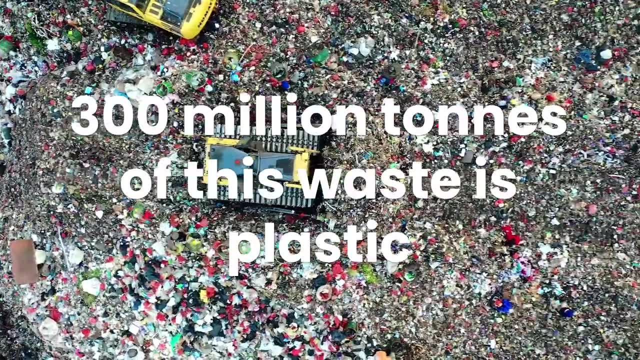 Globally, only 13% of all of our waste is recycled. Every year, humans produce more than 2 billion tonnes of waste. Nearly 300 million tonnes of this waste is plastic, and half of this is single use. Much of this ends up in landfills or even the oceans. 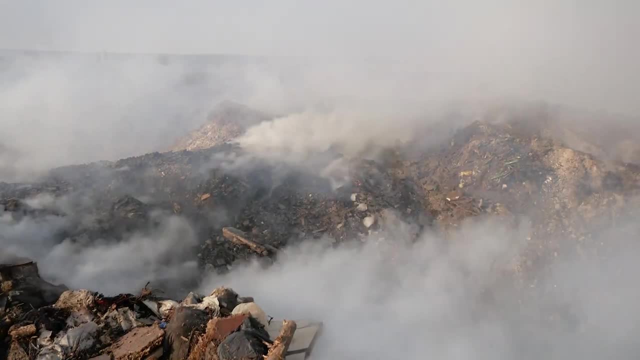 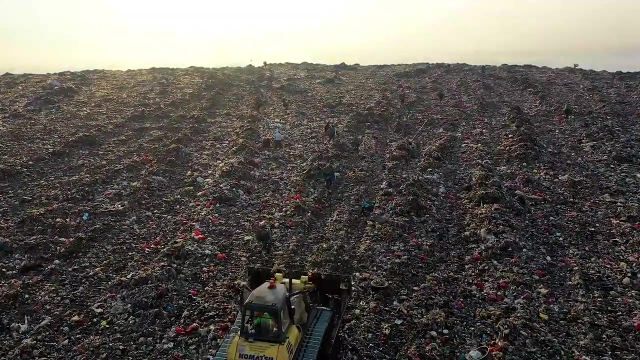 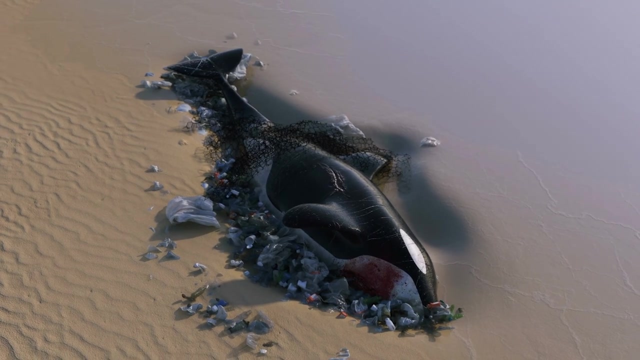 Landfills are one of the driving factors behind methane gas emissions, A powerful greenhouse gas that traps heat in the atmosphere, causing the acceleration of climate change. The waste that reaches the oceans is killing sea life due to the toxins in the plastics that enter the food chain. This, in turn, also threatens human health when 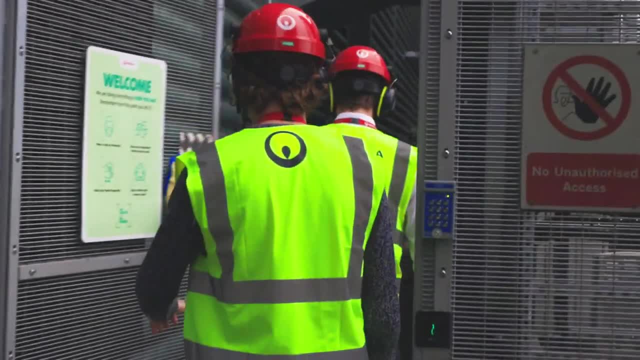 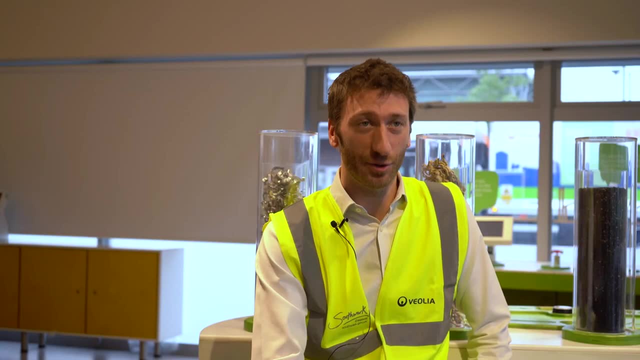 sea life is consumed. We sat down with the Director of Sustainable Technology at Veolia to get a better understanding of how important recycling really is. So my name is Tim Duretz, I'm a Director of Sustainable Technology, So I look after the improvements of 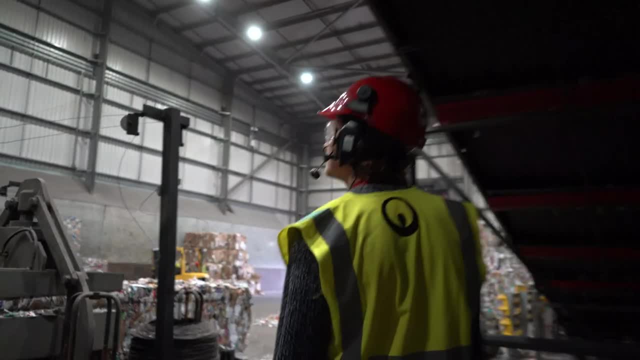 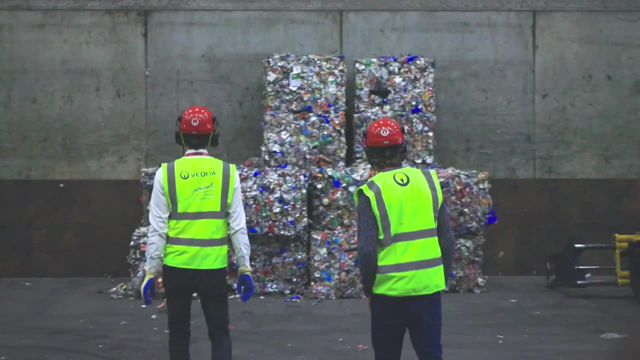 sorting and recycling for a company called Veolia, And we are collecting the waste of 6 to 8 million people in the UK, So it's called an integrated waste management facility. We are extracting the recyclable material: the plastic, the glass, the metal. 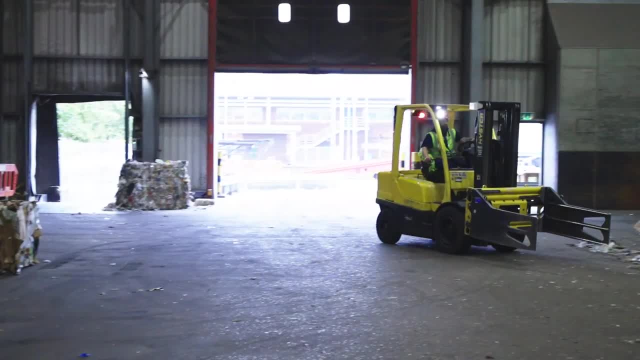 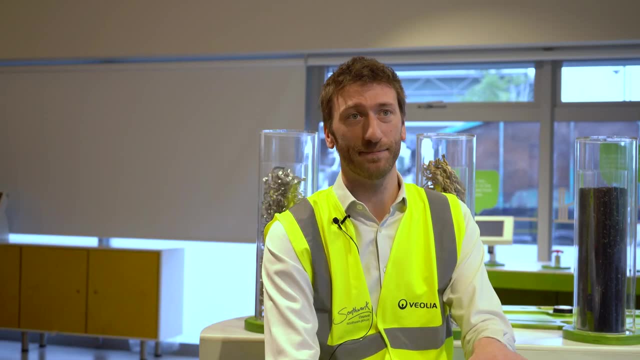 the fibre, the cardboard, etc. And it's about 120,000 tonnes per year, which makes it one of the biggest in the UK, But there are about 100 of these in the country. Recycling is when people put things into the bin without actually. 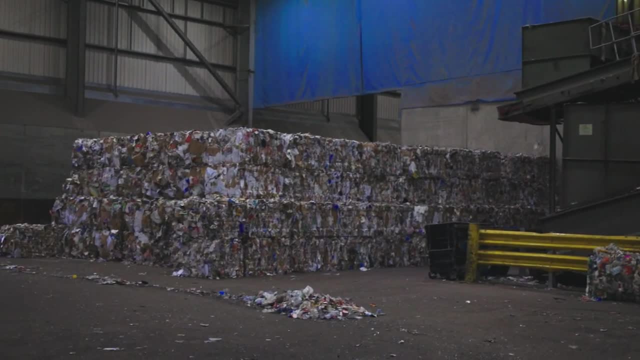 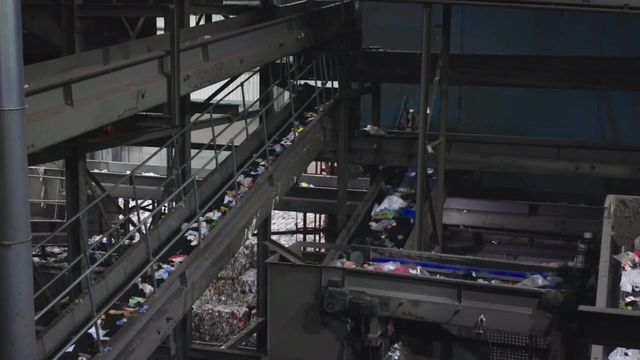 knowing whether or not it can be recycled. So we asked Tim how this has impacted the facility. It comes from a good intention. People want to recycle more, So they put things in their recycling bin which should not be there. The typical ones we've got are: 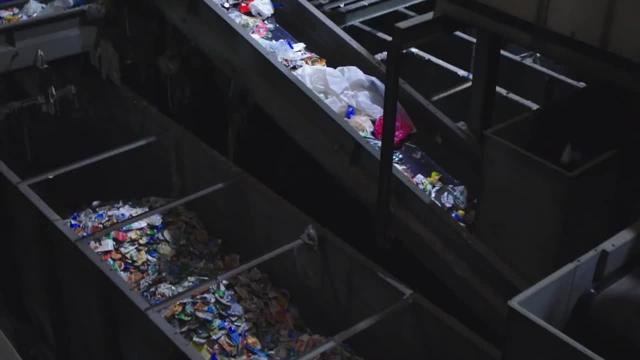 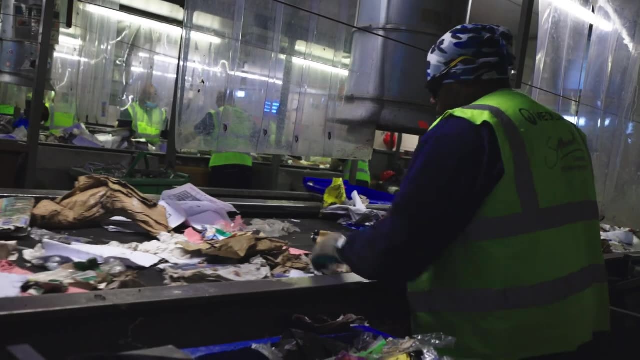 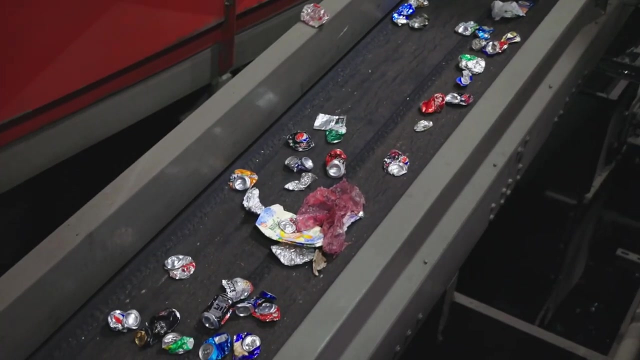 plastic toys, electronic devices. We can recycle them. We can collect them separately and recycle them, But not in the recycling bin. Different areas often have different recycling regulations, So we wanted to know why this is happening, For various reasons. One of the reasons is it has been 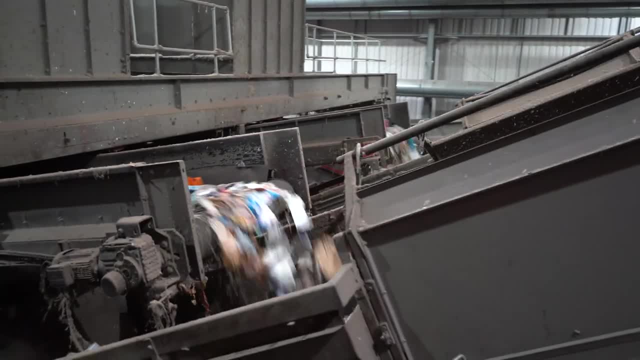 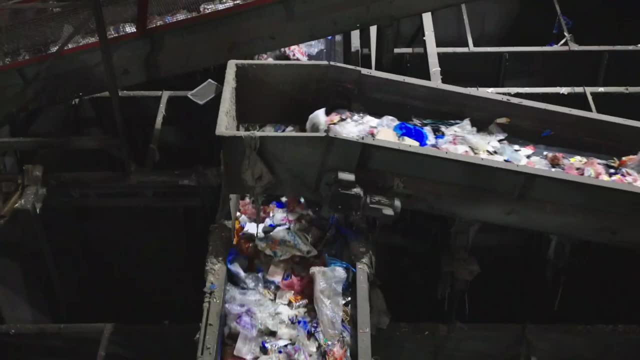 built 10 years ago. We might build a new one in the next few years, And the technology we use is different, has evolved, And that's why some can cope with certain plastics. But by 2023, 2024, there's a new governmental strategy. 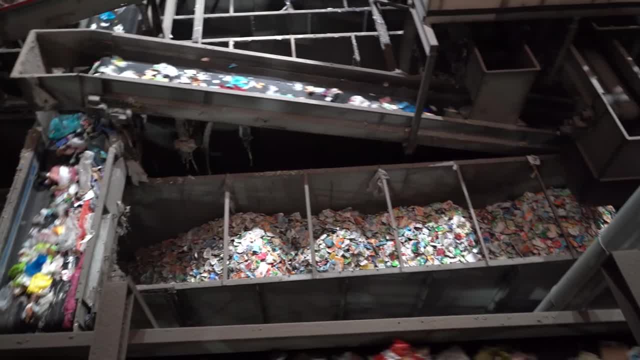 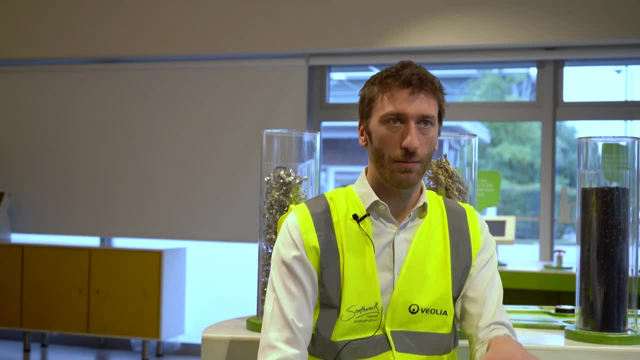 called the Resources and Waste Strategy. The aim is to harmonise that nationally. It's called Consistency of Collection. All the local authorities will collect the same waste. We need a bit of time as an industry to adapt, And we also talk about the labelling. So each 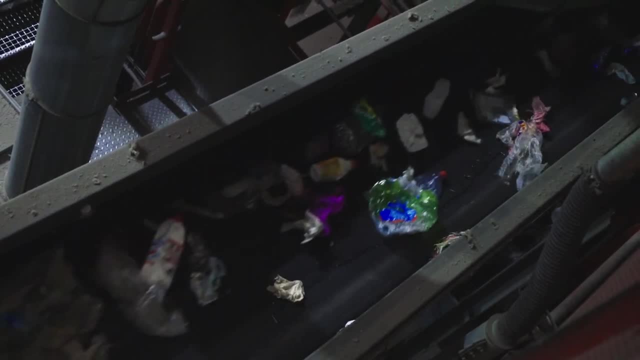 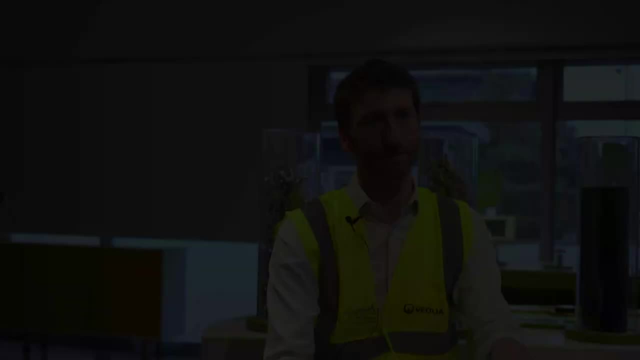 piece of packaging will have a standardised label which tells the public: yes, put it in your recycling bin, or no, put it in your rubbish bin. Lots of advancements are currently being made in the recycling sector, So we wanted to know if Tim was. 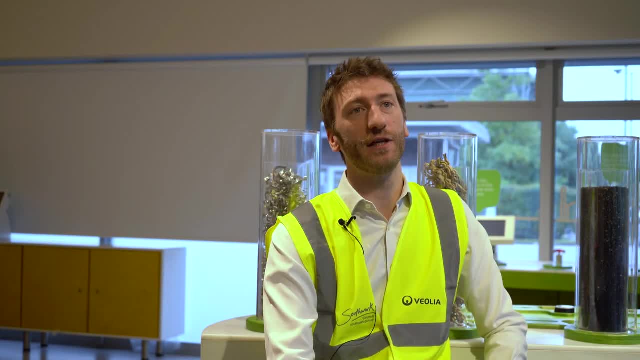 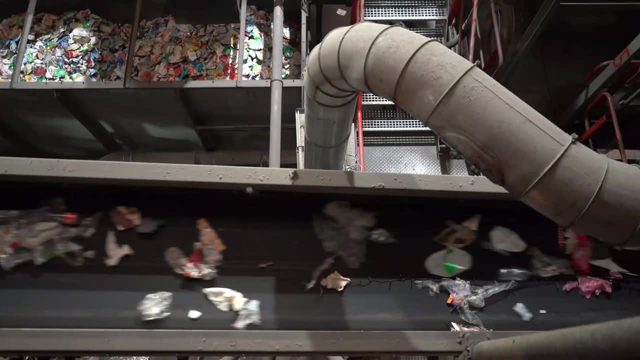 excited about the future. Yeah, very excited, and for different reasons. I think we've got more engagement from the public, New regulations coming, We've got the plastic tax, the deposit return scheme and the technology does evolve. You've seen on the side this artificial intelligence camera. 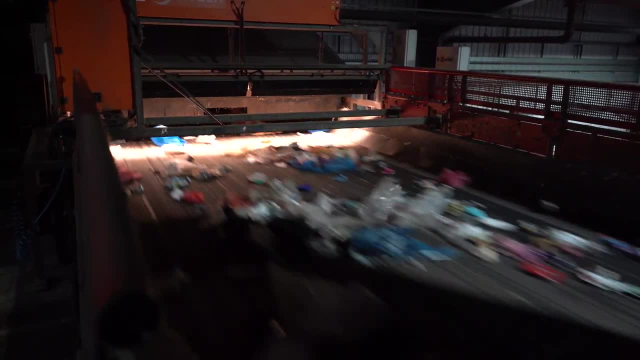 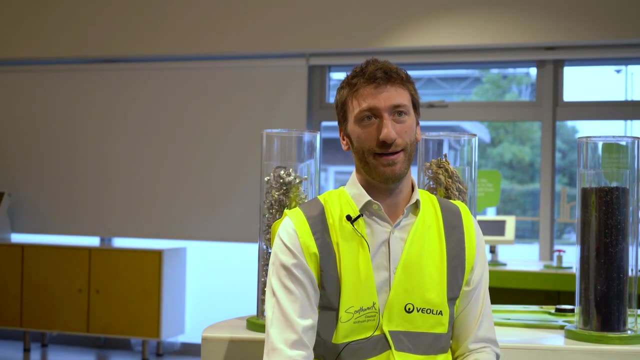 which is new, an innovation that we are doing as a company. So, all this together, I'm convinced that we will improve. So, yes, I'm hopeful and excited at the same time. Knowing what you can do at home can be challenging, So we asked Tim for his 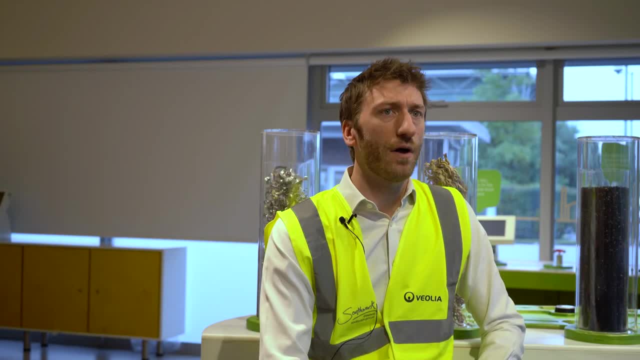 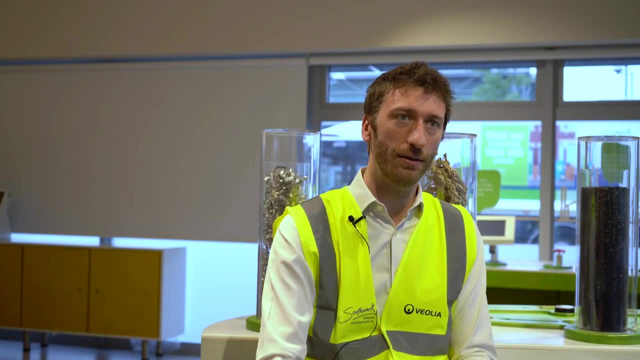 main piece of advice for the public Probably to follow the guidance. You know, if you go on your council's website, you will find a section about recycling what can go in your recycling bin. So that would be number one. And number two is when you go shopping, you know, there's the eco-design. 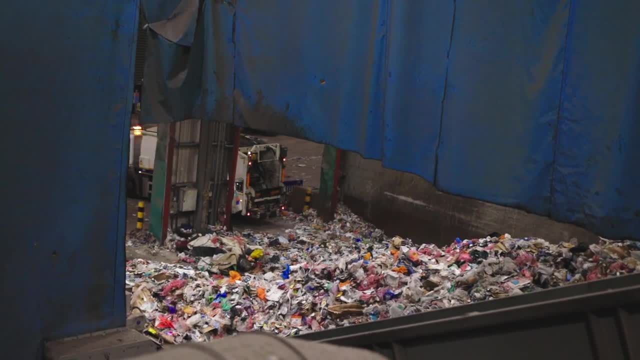 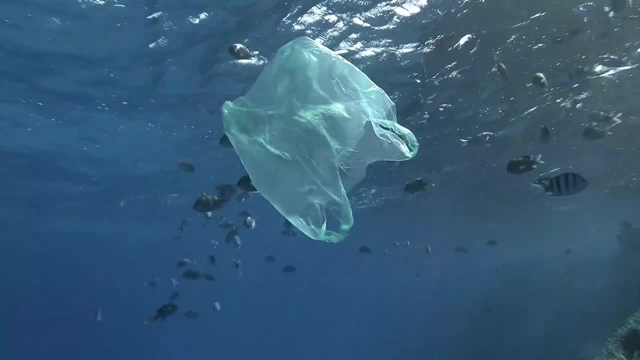 packaging, So when you buy, you know you've got the power to change and to help the recycling rate of the country when you purchase your goods. Soft plastics are one of the main issues affecting sea life, So we wanted to know why. 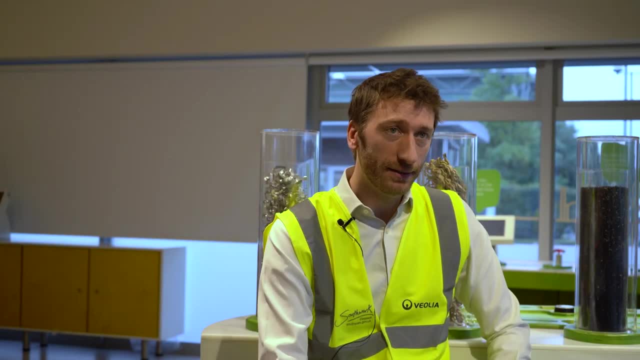 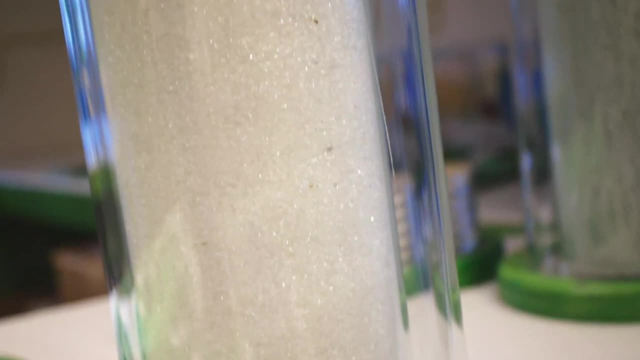 Why they weren't being recycled more. The main reason is it's not easy to sort out the other waste. It's also quite expensive to recycle it. to make you know pellets that we do out of bottles And it's a bit more difficult. 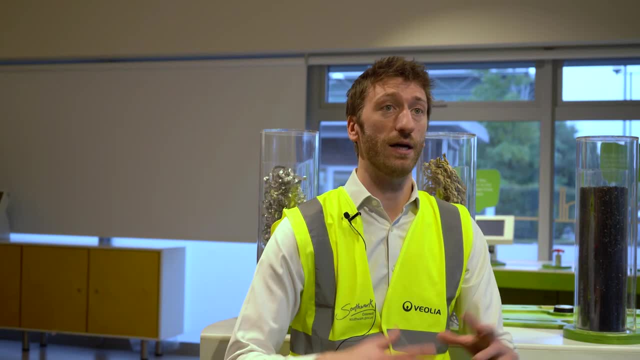 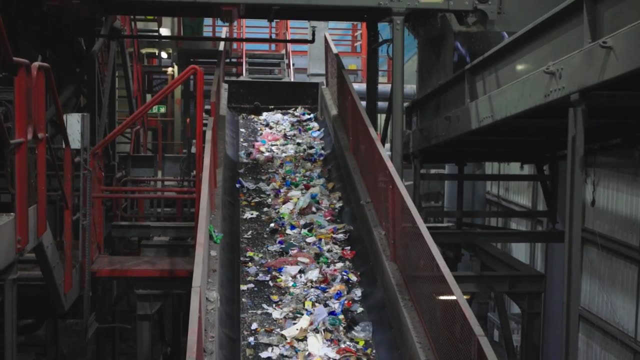 to do with soft plastics. That's why some supermarkets decided: okay, I'm going to collect it in front of stores, Then it's clean, it's isolated, and then it's easier for a company like Veolia to then recycle it. So we're trying. 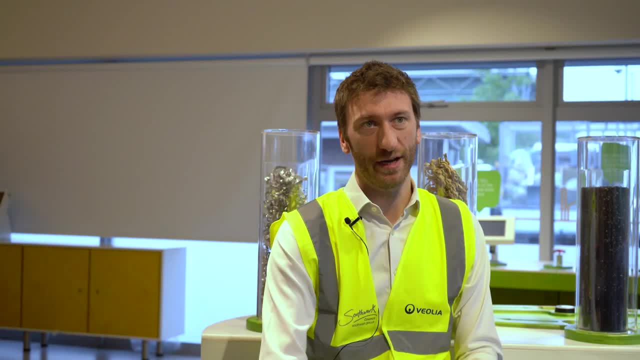 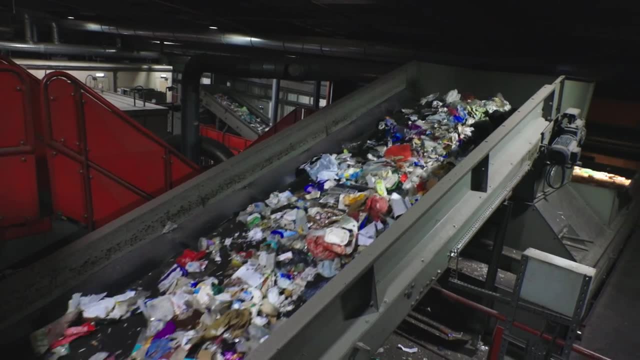 but ideally it needs to be collected Separately. But again, at the end of the day, I think we know how to recycle. This is happening And what we need to do is to do more of this, To have more of this facility. 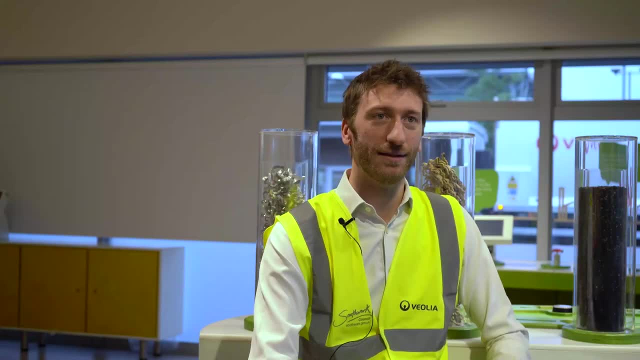 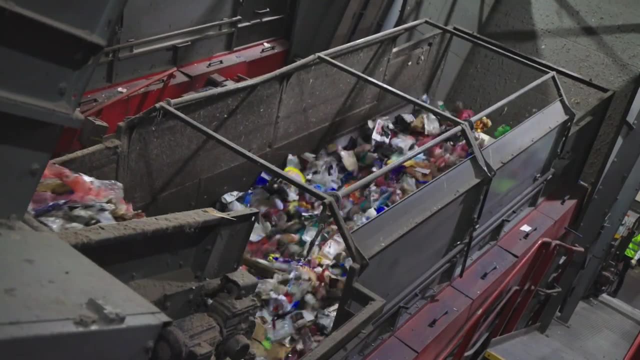 and to do better at the country, And let's do it. We should all try and be mindful that once we're done using something, it goes on a journey and becomes someone else's responsibility. We hope you are able to have a greater understanding as well as. 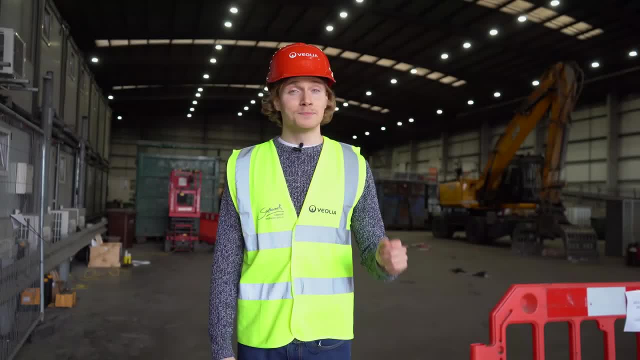 take some tips from this video and apply them in your daily habits. Please give this video a thumbs up and subscribe if you want to see more videos like this. Thank you very much for watching and we'll see you in the next one. 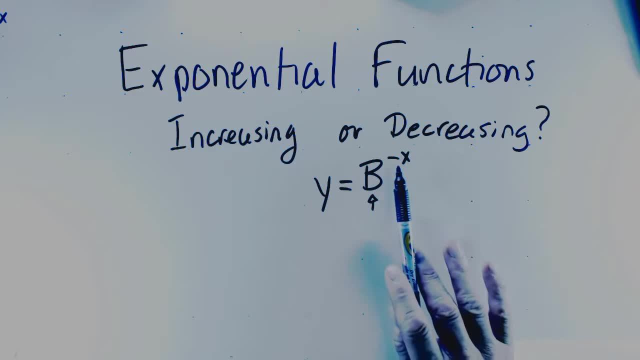 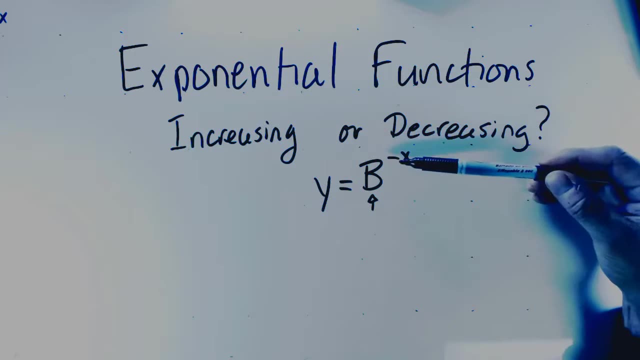 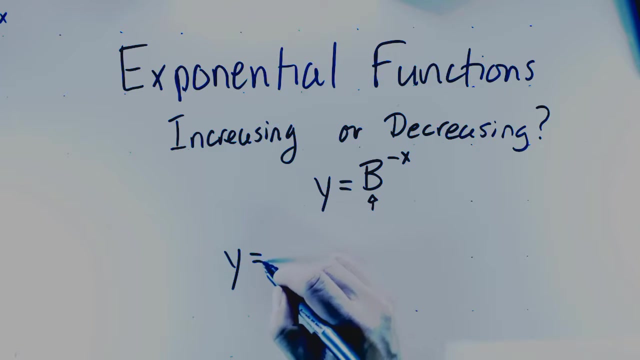 Now what if we have a function that is some base to the exponent negative x? Is that increasing or decreasing? We just have to remember that this negative x means reciprocal, and so essentially, functions that look like this- y equals one half to the exponent negative x- are the same. 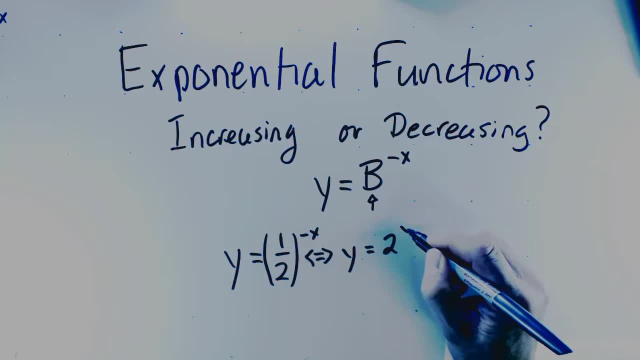 as y equals two to the exponent x, And so a function that looks like this is equivalent to a function that looks like this, and so this function is going to be increasing as we move from left to right, in other words, increasing through it's domain. If, on the 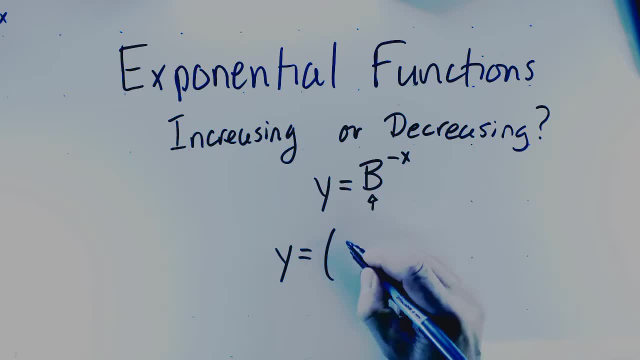 other hand, we have a function that looks like this: y equals three halves to the exponent, negative x. In this case, you will notice that the base is greater than the exponent, greater than 1, and this is a negative x, and so that means take the reciprocal. 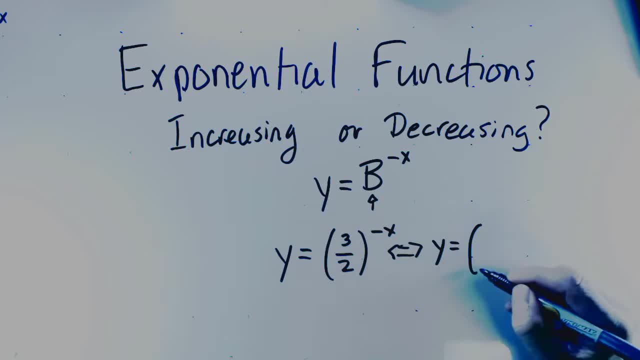 So this is essentially equivalent to y, equals 2 thirds to the exponent x, And so this function- because the base is actually between 0 and 1, is going to be decreasing throughout its domain, And so the reciprocal property actually tells us what happens relative to the increasing.